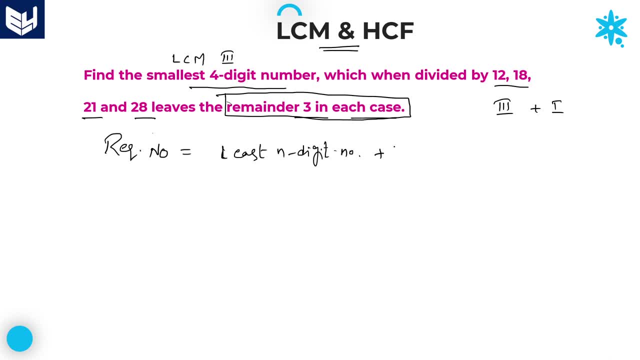 and digit number LCM minus remainder. Up to here this is third model and after that if it is a combination of three and one, whenever that particular problem belongs to third and one combination, in that case, whatever the remainder which is given in the problem, let us consider that. 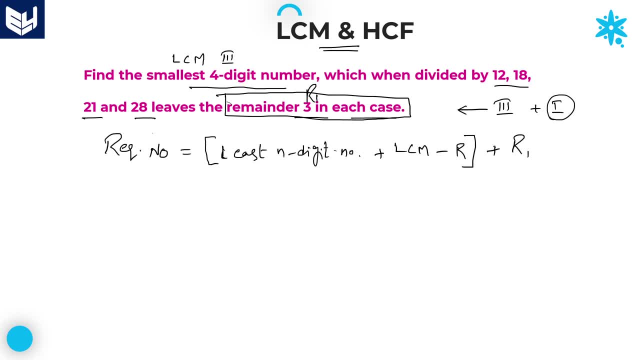 remainder as R1.. You need to add that remainder, also R1.. This remainder is different and this remainder is different Here. R1 is the remainder which is given in the problem, where R is the remainder obtained by dividing least and digit number. 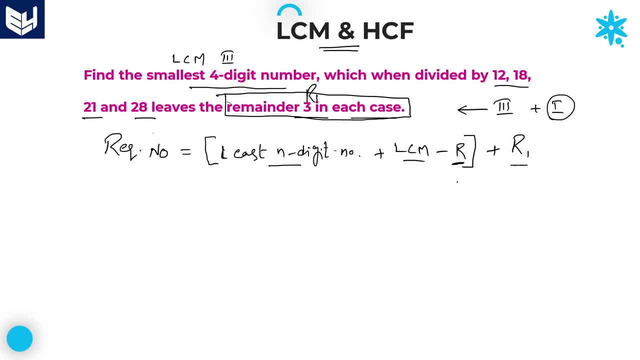 with LCM. That is the difference between these two remainders. Now here the least and digit number. As we are talking about least four digit number, So least four digit number is 1000 plus. After that we need to calculate the LCM. Here the numbers are 12,, 18,, 21,, 28.. Calculate the LCM of these. 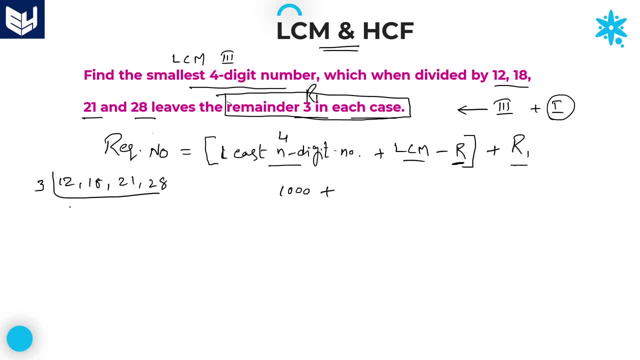 four numbers I will take with 3.. 3, fours, 3 sixes, 3 sevens, and it is not divisible by 3.. After that you can go with 2.. 2, twos, 2, threes, 7,, 2 fourteens. Next again you. 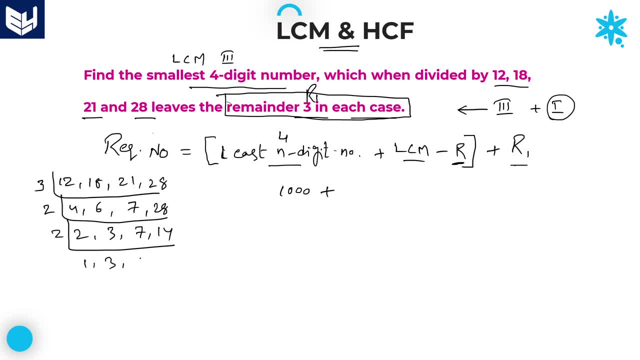 can go with 2, 2 oneses, 3 sevens and 2 sevens. Now you can go with 7, 1, 3, 1, one time. Now the LCM of all these numbers, all these four numbers, LCM is equal to how many threes? 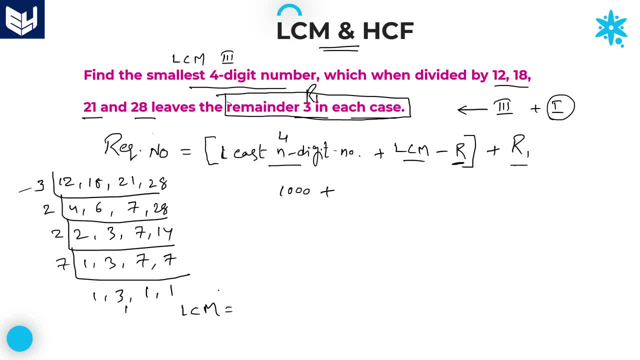 are there 1,, 2, 2 threes? How many twos? 2 twos, 2 square into 3 square into 7.. This is the required LCM. 2 square is 4 and 3 square is 9.. 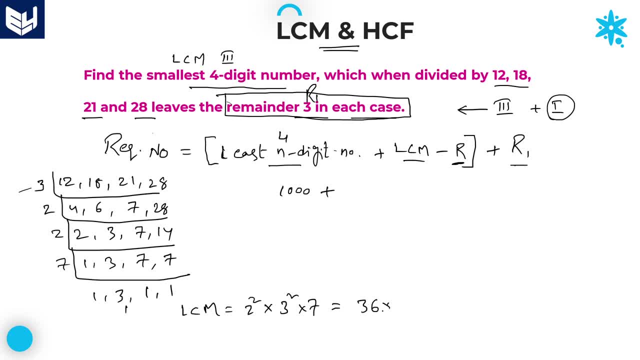 4 into 9, 36.. 36 into 7.. We need to calculate this value Here. it is 30 into 7, which is equal to 210.. 210 plus 42, that is 240, 252.. LCM of all these numbers is 252.. 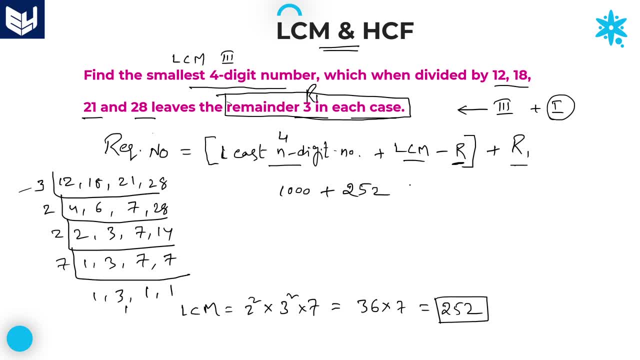 And substitute that LCM over here 252.. Now you can divide this least 4 digit number with LCM. What is LCM 252.. Here it is 3 times 756.. 756.. And if you take 4 times it will cross 1000.. 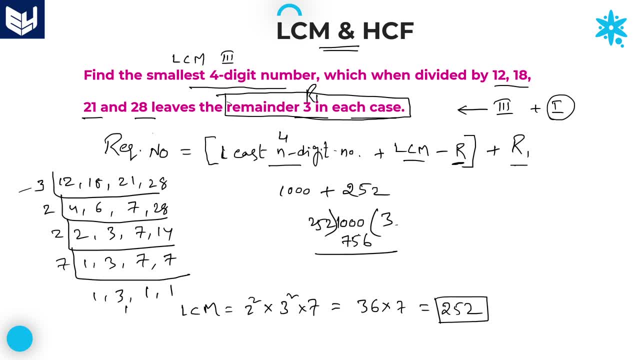 So it is only 3 times 252, 3 is 750.. Now you can subtract these two. What you will get is: here it is units, plus is 4.. And 1000 minus 256, which is equal to: here it is 244. 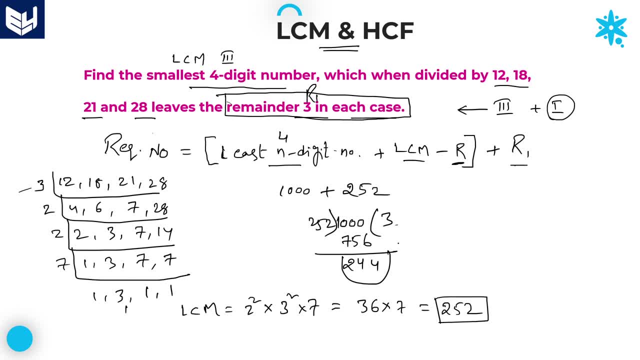 The remainder which we are obtaining is 244.. That remainder should be subtracted from this LCM Minus 244, plus whatever the additional remainder which is given in the problem That You need to add Plus 3.. Here, if you take the difference between these two, 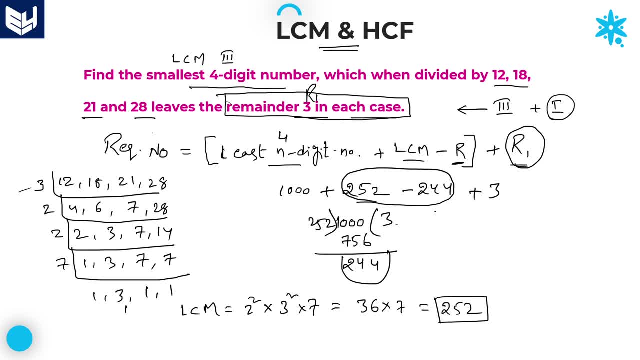 252 minus 244, which is equal to 8.. Which is equal to 8.. 8 plus 3, 11.. 1000 plus 11.. Which is equal to 1011.. Here our required answer for this question is 1011.. 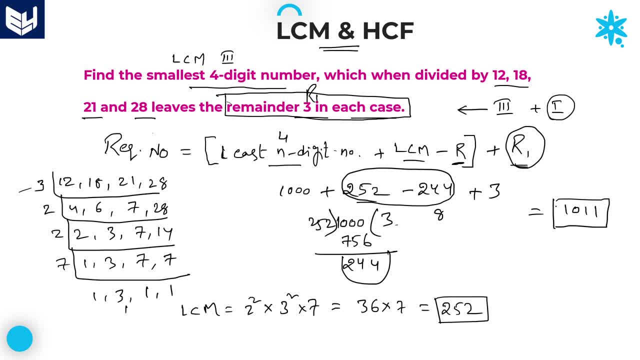 Here. the meaning of exact meaning of this particular question is: 1011 is the smallest 4-digit number which, when divided by 12,, 18,, 21,, 28,, leaves the same remainder 3 in each case. That is the meaning of this particular question. 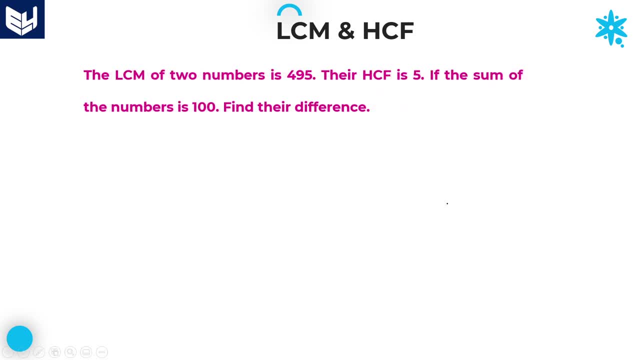 I hope you understand. Let's move on to the next question. See here, The LCM of two numbers is 495.. The LCM of two numbers is 495.. And their HCF is given as 5.. And their HCF is given as 5.. 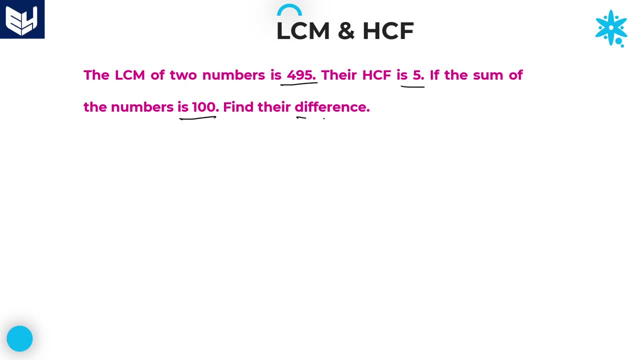 If the sum of the numbers is 100, then find their difference. If the sum of the numbers is 100, then find their difference. Guys, in LCM and HCF topic, whenever HCF, of any two numbers are mentioned, then we have to consider those two numbers must be a multiple number. 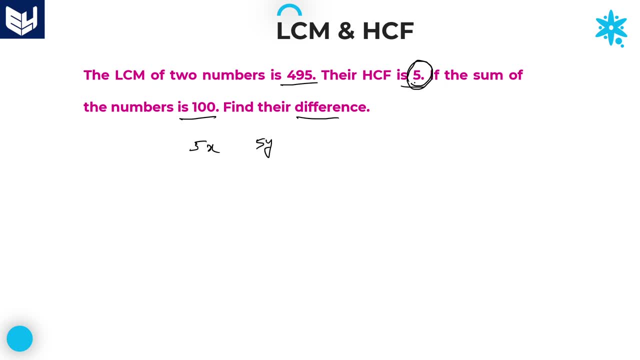 That is why in LCM or LCD the number of numerals must be a multiple of HCF. Here, if HCF is 5, then definitely those numbers are multiples of HCF. Why? because if those numbers are not multiples of HCF it is not possible to get the HCF as 5.. 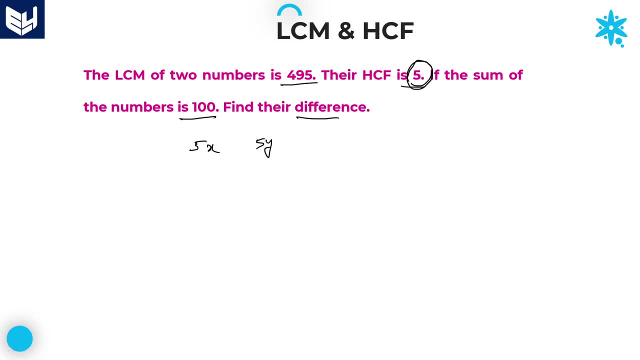 That is the reason why, whenever two numbers- HCF- is given, you need to take the multiples of HCF, only those numbers. Let us take two numbers: 5x and 5y. According to the given conditions and information, LCM of two numbers is 495.. 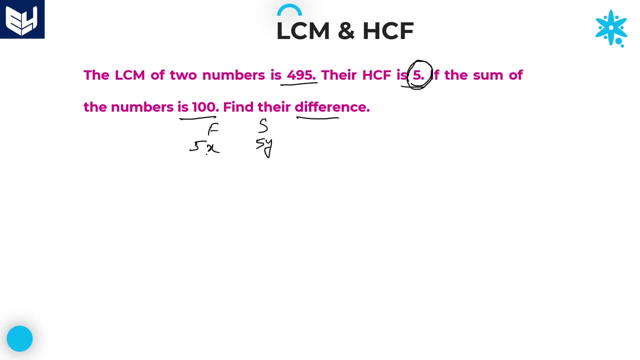 This is first number and this is second number: LCM of these two 5x and 5y. LCM is LCM of 5x and 5y, which is equal to 5xy right. That value is given as 495.. 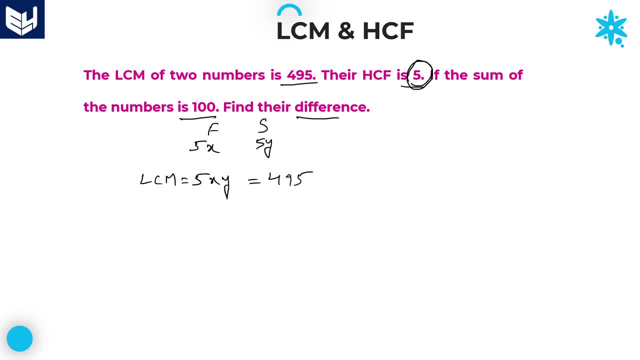 5xy is equal to 495.. Now you can cancel with 5 table. 5 x 9 is 45.. Again, 4 is there. 45 means 5 x 9 is 45.. x into y is equal to 99.. 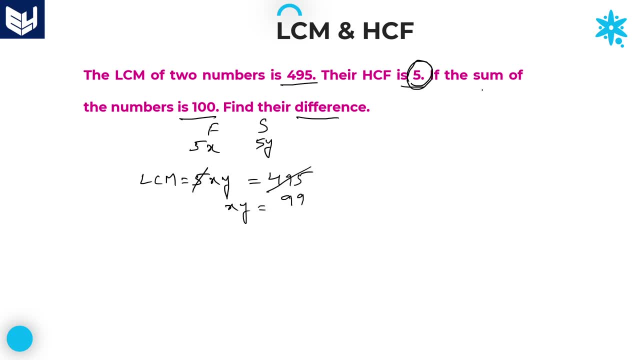 x into y is equal to 99.. One more information is also given, That is, sum of two numbers is 100.. Here the two numbers are 5x and 5y. Sum of these two is equal to 100.. 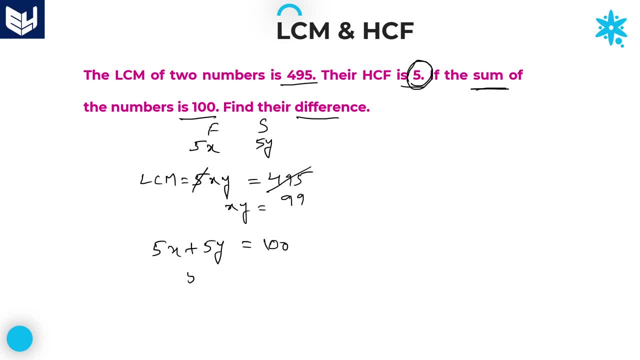 Sum of these two is equal to 100.. Now you can common 5.. 5 into x plus y, which is equal to 100.. 5 x 1 is 5 x 20.. So x plus y is equal to 20..